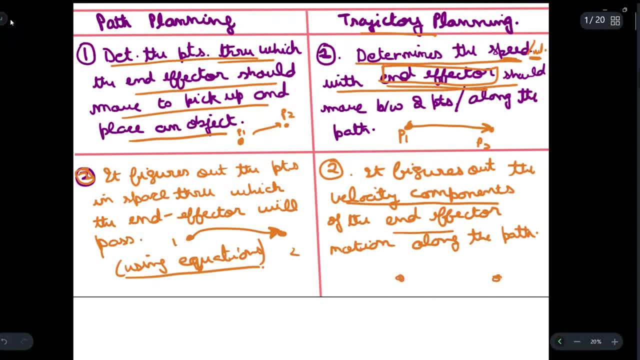 trajectory planning. we will try to optimize the path planning, that is, we can say that path planning is the simplest part. that is, just finding out the path based on car. stopped are гл다 To corrections r, b. it is not defined as the confused path. E and J are Ferrari p, 2 for E and R are for E and R are for P and p 2 for A and P and stop are P, or R are for P, 5 for E and Cm for V. so P 1 for P and P and P and P 3 are for E and P 3 are for P. We will get that one difference in� altro as a. 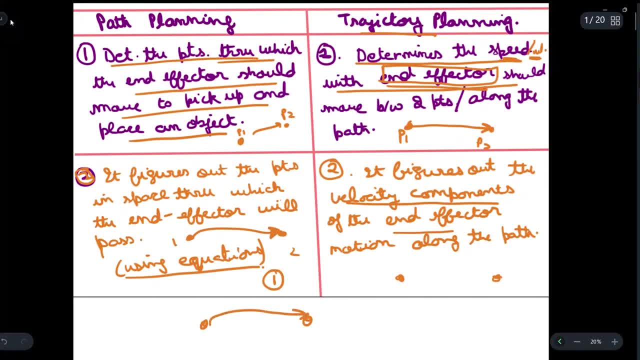 path through which the manipulator should travel, and in trajectory planning we will determine the speed, the time and the velocity with which the manipulator should move in order to find an optimal path. so trajectory planning is necessary in order to easily move a manipulator from one point to another or to place an object from one point to another. 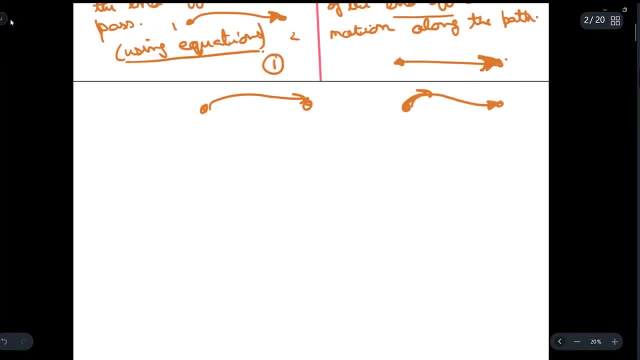 so now we will discuss the parametric form of both of these plannings. that is, suppose we have two points, that is, x1 y1 and x2 y2, and we have to go from x1 y1 to x2 y2. so in 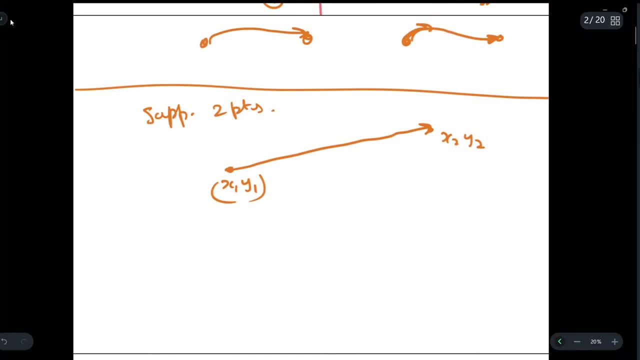 order to do that, we will first of all write the parameters for path planning in parametric form, that is, this one is for path planning. okay, so the first parameter for x will be v into x1, x2 minus x1 upon x2 minus x1, whole square. 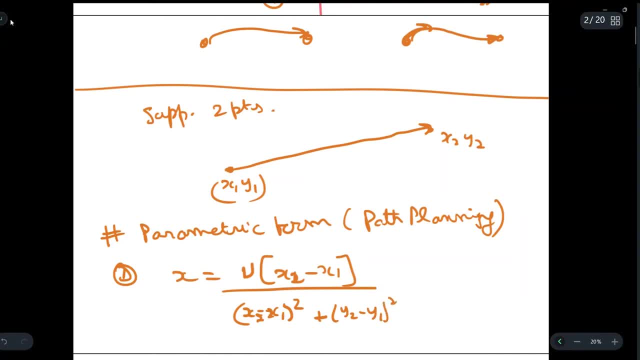 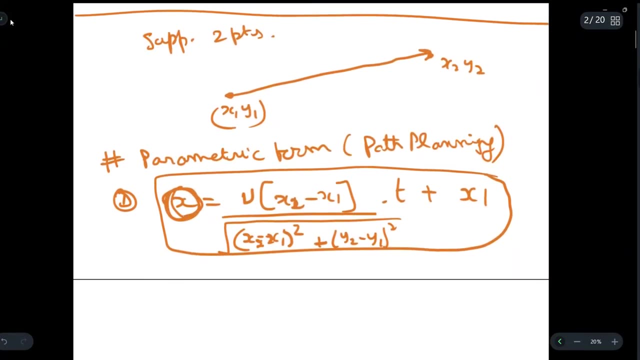 plus y2 minus y1, whole square and every, everything into the under root, into t plus x1. so this is the parametric form, that is, this is the coordinate, this is the position or the coordinate of the manipulator which we can find at any given time. t and v is the. 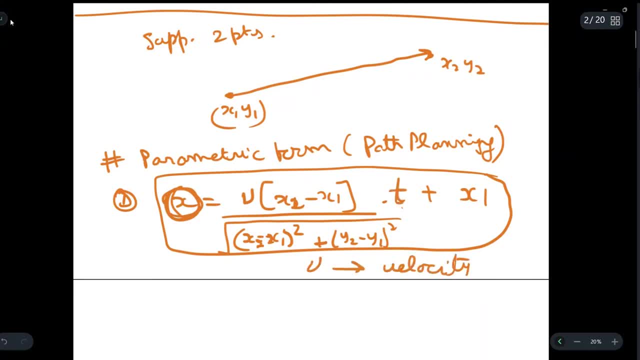 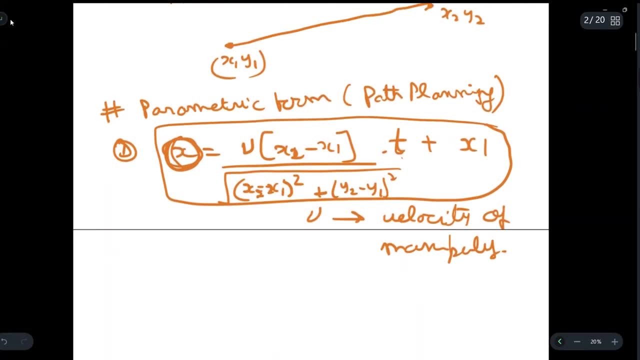 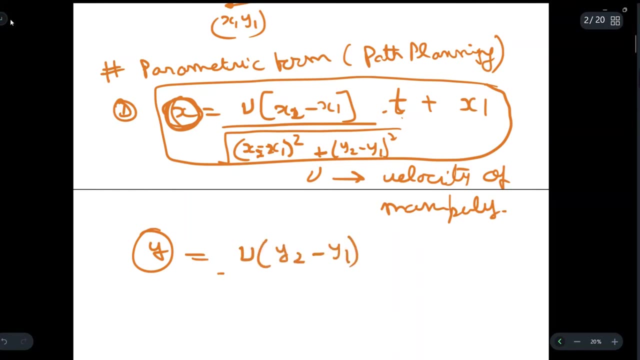 velocity over here, that is the velocity of the manipulator. now, similarly, we have another equation in parametric form with respect to y, that is, it will be given by v into y2 minus y1, upon x2 minus x1, whole square, plus y2 minus y1, whole square, and every everything into 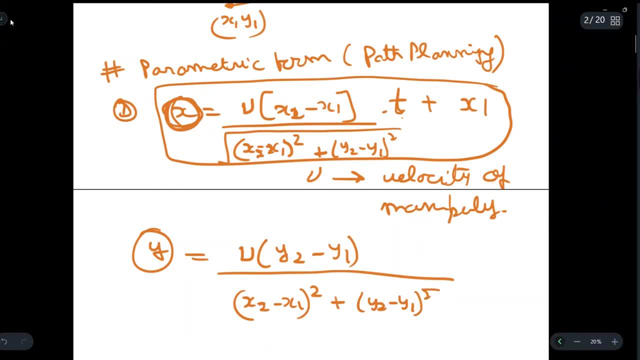 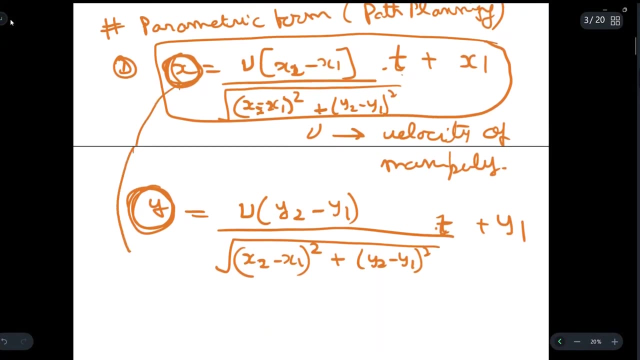 t force, okay, whole square, and to the under root, into t plus y1. so this is the y coordinate or the y position which can be found out at any given point. t at any given time, t, that is. these two will be the coordinates of the end effector. 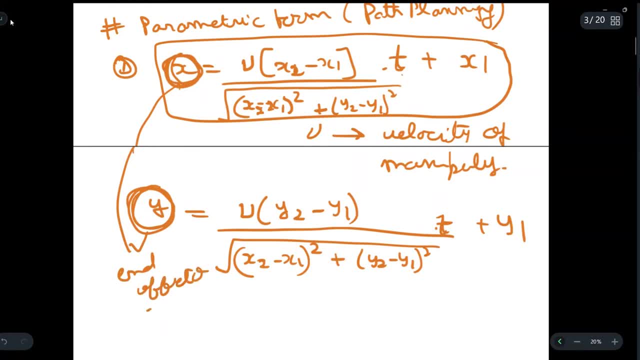 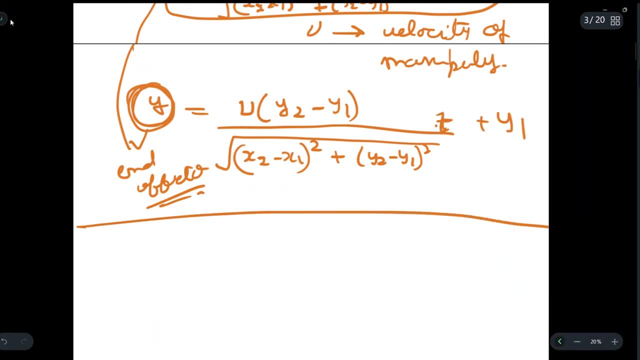 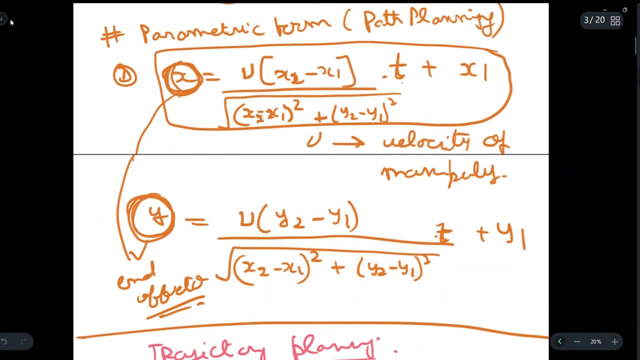 this is done in path planning. now, in second part, let us come to the trajectory planning path. in trajectory planning, we will all we also have certain parameters. that is, we will simply differentiate. differentiate the x coordinate that we found over here. that is, on differentiating, you will get v into x2 minus x1. 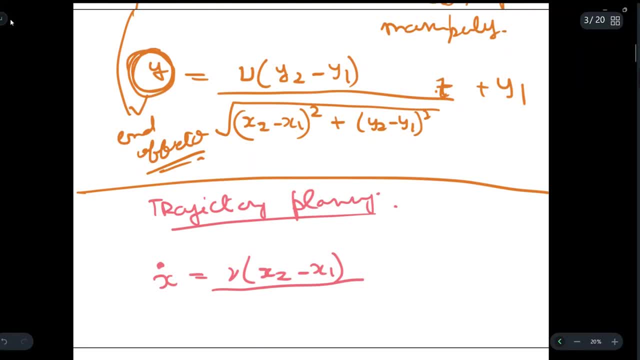 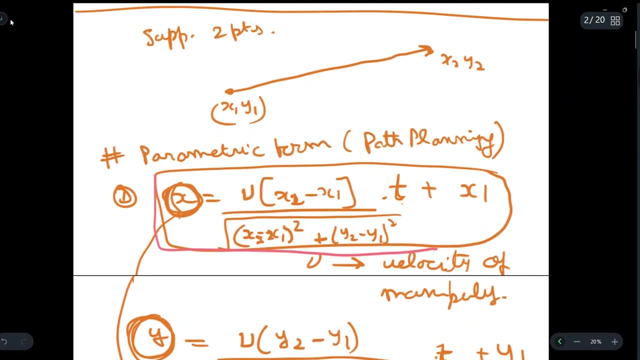 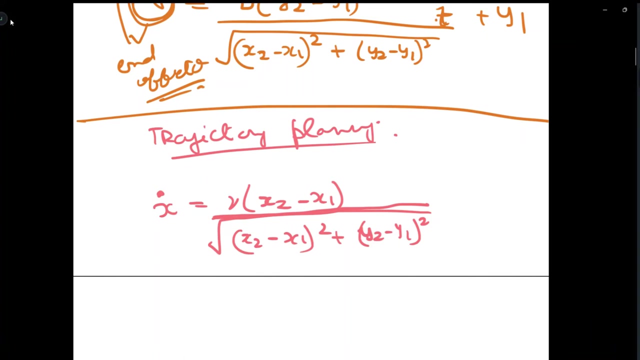 upon x2 minus x1 whole square plus y2 minus y1 whole square and everything to the under root. here we have differentiated the path planning parameter by t, that is, we have differentiated this by t, so we have got the value, as x dot is equal to v, into x2 minus x1 and under root upon. 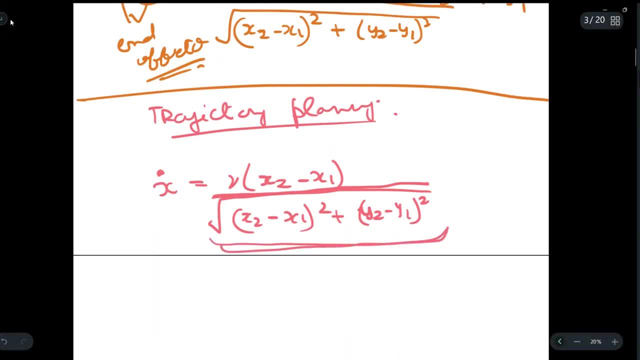 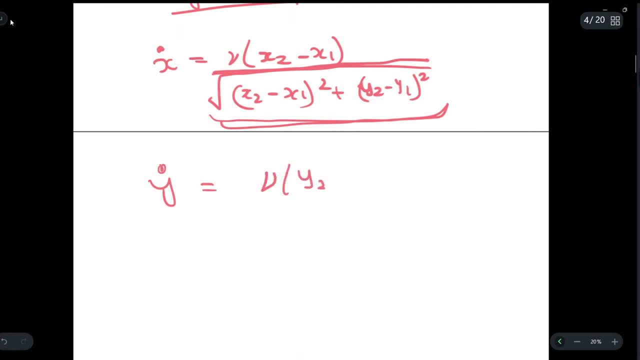 this now similarly. similarly we will find out for y, that is, we will get y into y2 minus y1 and upon x2 minus x1 whole square plus y2 minus y1 whole square to the under root. so these are the parametric form for a trajectory planning. 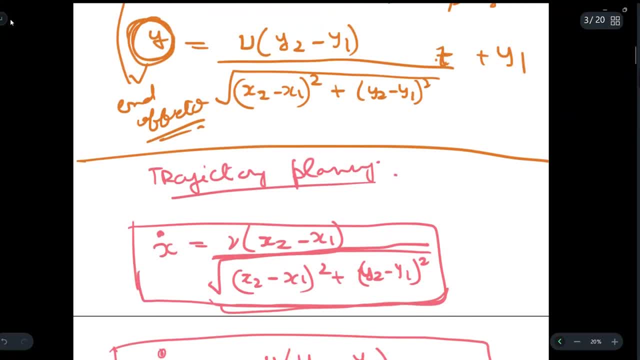 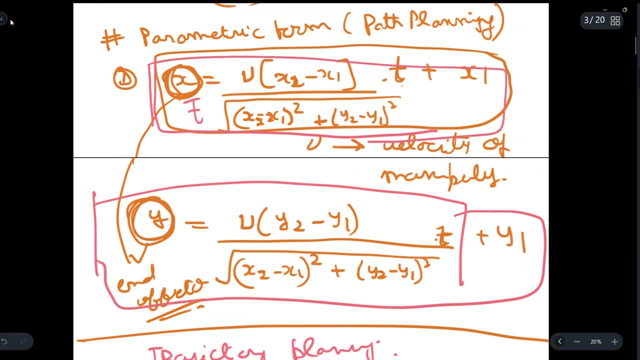 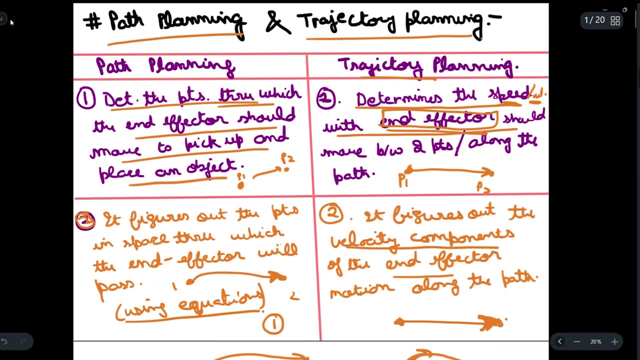 and these. these are the coordinates. sorry, these are the coordinates for the path planning. so these are two parameters that we need to find out. so i'll again brief up what i just said: in path planning, we just have to find the path between two points, irrespective whether it is. 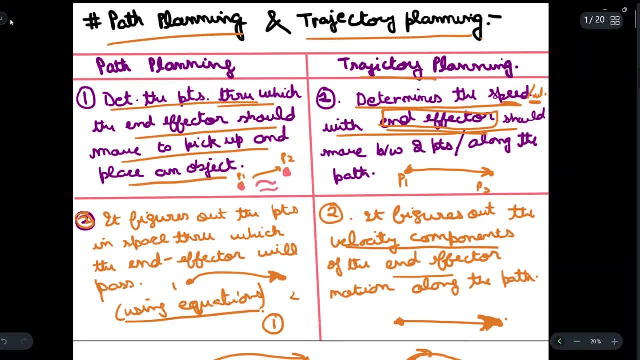 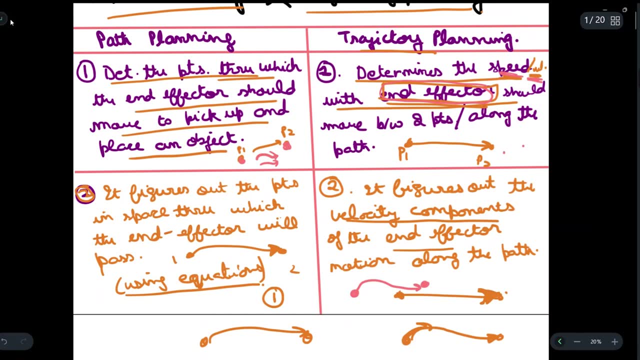 optimized or not, and we do not consider the velocity or the force over here, whereas in trajectory planning we not only consider the path that we got from path planning, but along with that we also consider the speed and the velocity with which our end effector should move from one point to another. so this 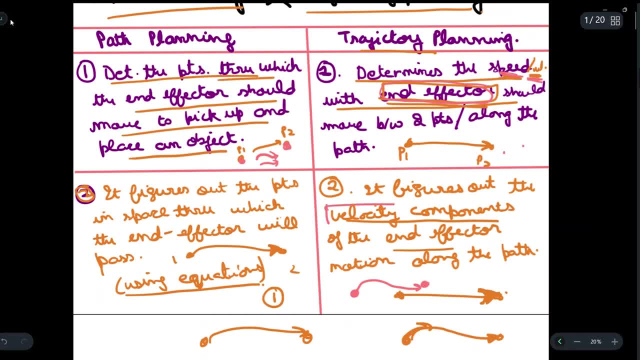 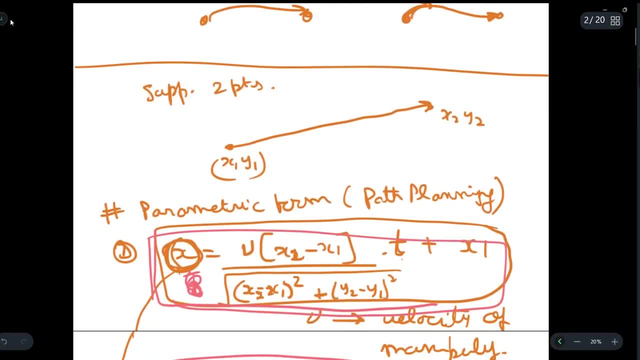 is the main difference between the two. in this we find out the velocity components and in this we figure out the points in space through which the end effector should pass. now, this is it for this video. if you were able to understand this video, just write in.